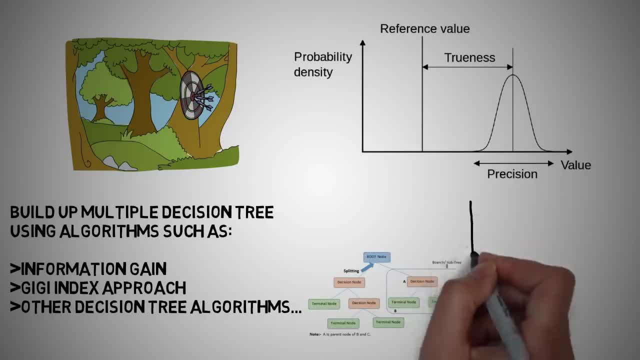 other algorithms. If you are not aware of the concepts of the decision tree classifier, please check out my other lecture on decision tree got for machine learning. You will need to know how the decision tree classifier works before you can learn the working nature of the random forest algorithm. 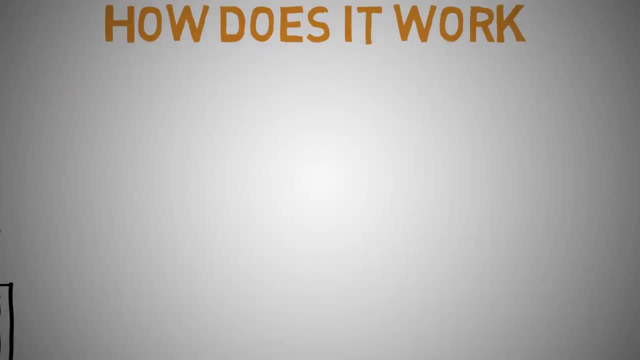 So how does it work? In random forests we grow multiple trees as opposed to a single tree. in the cart model To classify a new object based on attributes, each tree gives a classification and we say the tree votes for that class. The forest chooses the classification having the most votes over all the other trees in. 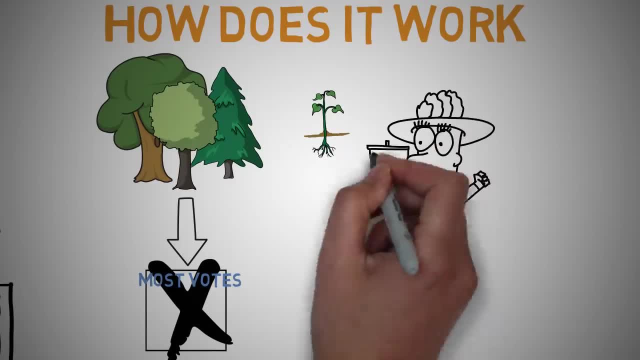 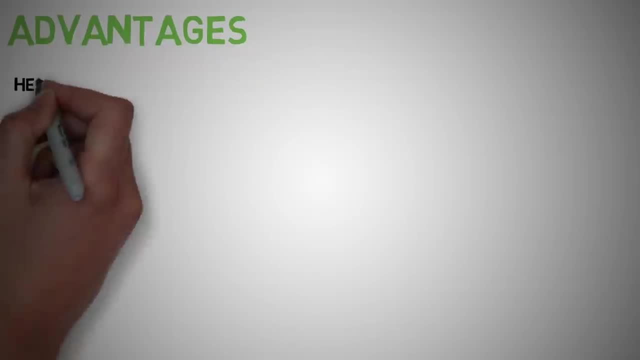 the forest And in the case of regression it takes the average of the outputs by different trees. So let's look at the advantages of the random forest 1.. So the same random forest algorithm or random forest classifier can be used for both classification. 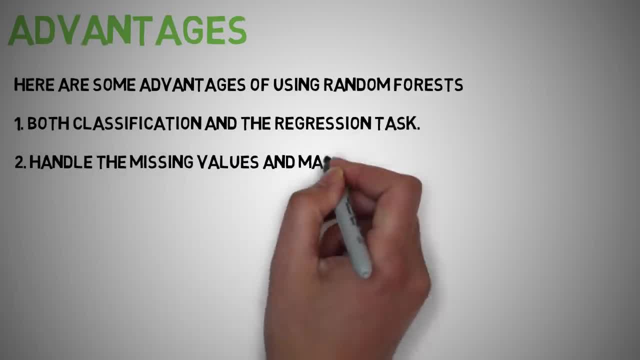 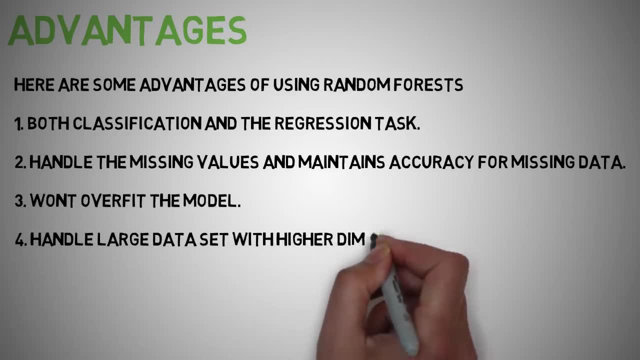 and regression tasks. Random forest classifier will handle the missing values and maintain accuracy when a large proportion of the data are missing. When we have more trees in the forest, random classifiers won't overfit the model. It has the power to handle large datasets with higher dimensionality. 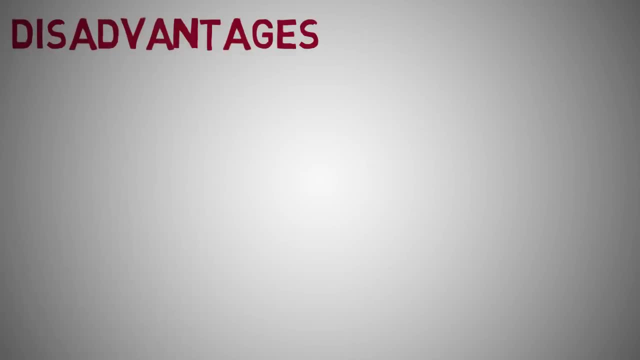 If we look at the disadvantages of random forest, however, It surely does a good job at classification, but is not as good as for regression problems as it does not give precise, continuous nature predictions. In the case of regression, it doesn't predict beyond the range of the training data. 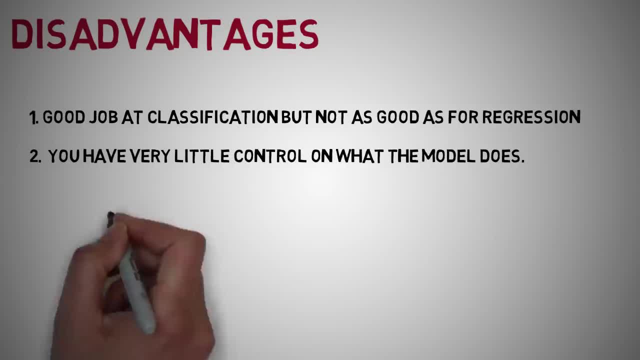 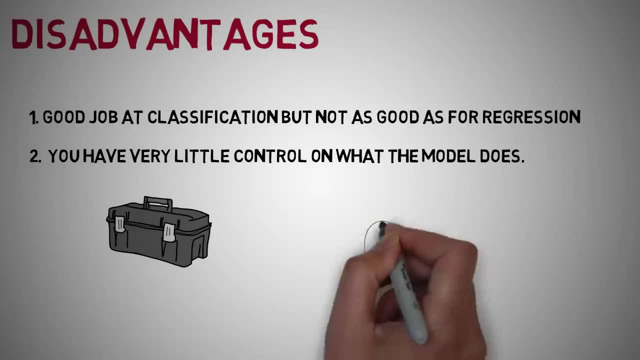 And they may overfit datasets that are particularly noisy. Random forest can feel like a black box approach for statistical modelers. You have very little control of what the model does. 2. Random forest classifier can be used to test different parameters and random seeds. 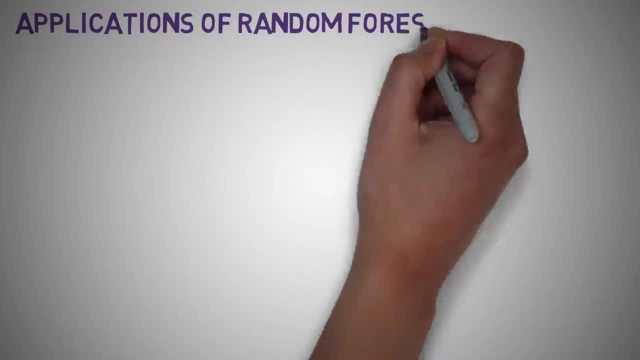 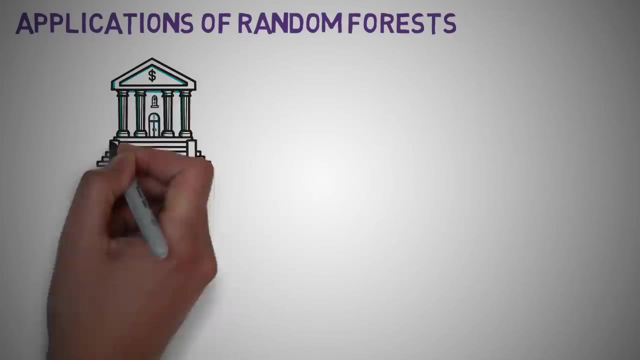 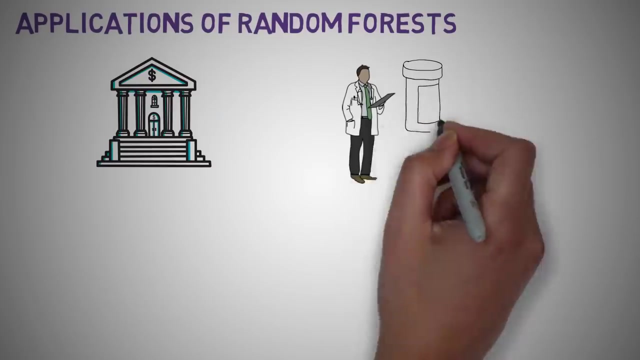 So what are the applications of random forest? So let's check a few of them down below So we can use them in the banking sector. So these are for finding loyal customers and finding the fraud customers. It can be used in medicine, where we identify the correct combination of components to validate. 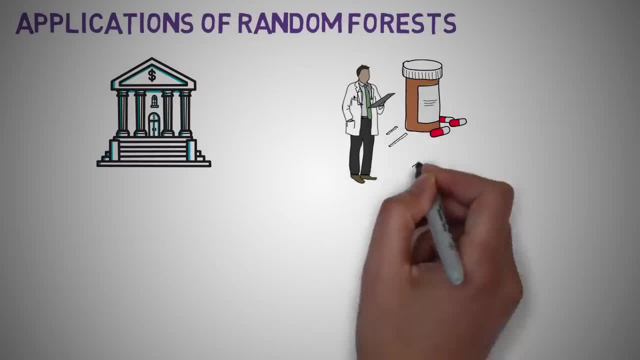 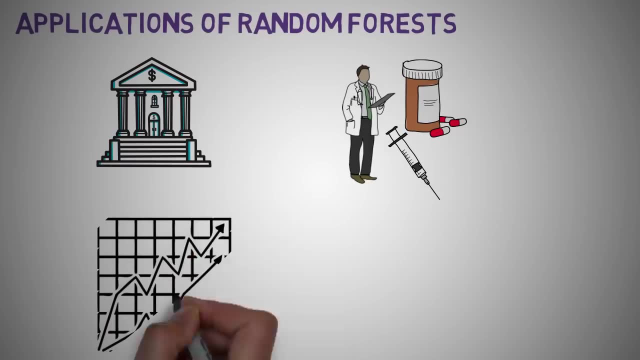 medicine. Random forest algorithms are also helpful for identifying disease by analyzing the patient's medical records. In the stock market, random forest algorithm is used to identify the stock behavior as well as the expected loss or profit by purchasing a particular stock. In e-commerce, the random forest is used in a small segment of the recommendation engine. 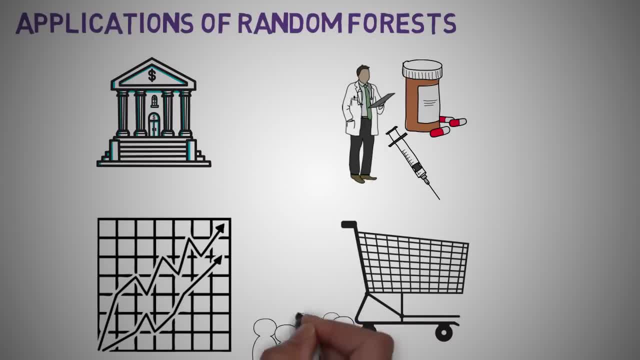 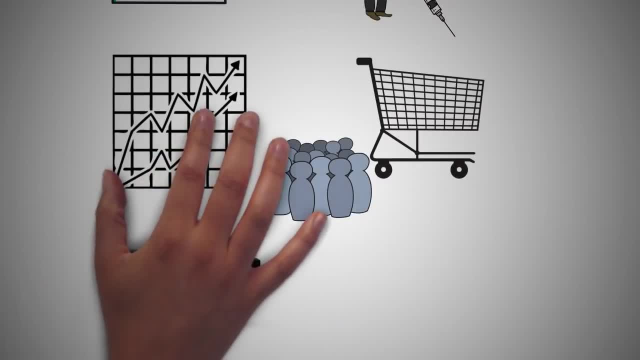 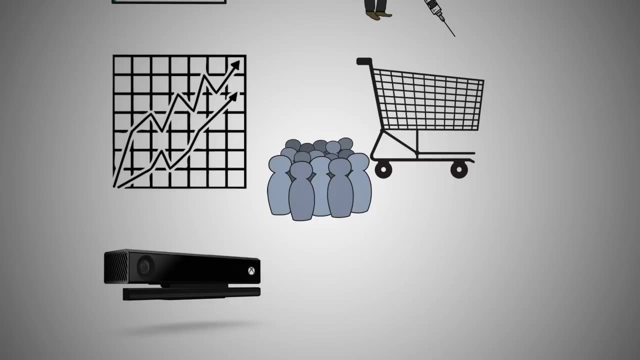 for identifying the likelihood of a customer liking the recommended products, And this is based on similar kinds of customers. In computer vision, the random forest is used for image classification. Microsoft has used random forest for body part classification for Xbox connect And other applications involve lip reading as well as voice classification. 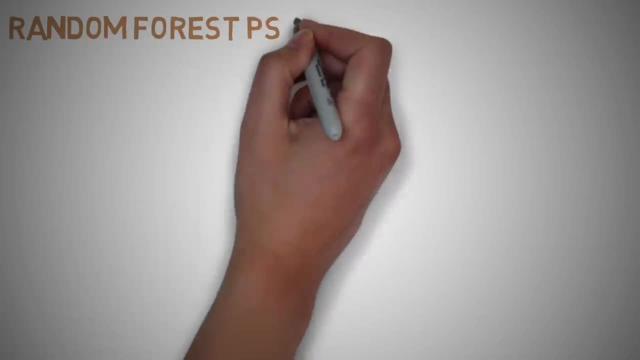 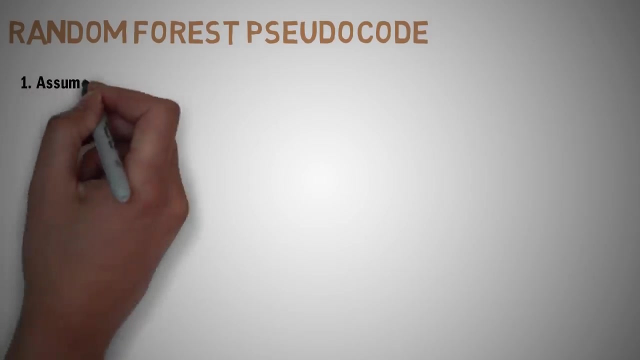 Let's take a look at the random forest pseudocode and how it works. So it works in the following manner: where each tree is planted and grown as follows. So assume a number of cases in the training set is N, Then the sample of these N cases: 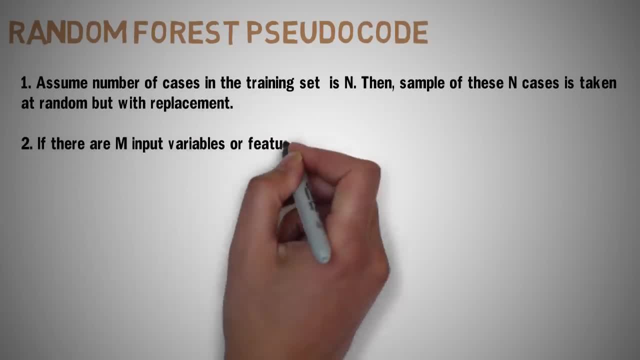 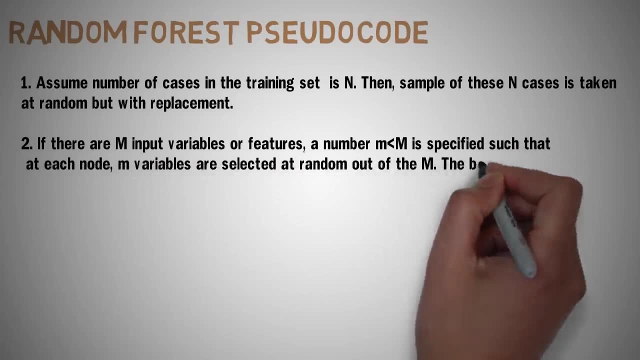 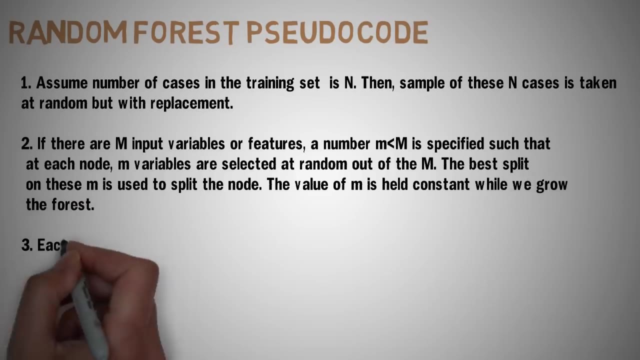 is taken at random. But what replacement? The sample will be the training set for growing the tree. If there are M input variables or features, a number of M smaller than M is specified, such that each node M variables are selected at random out of the M. 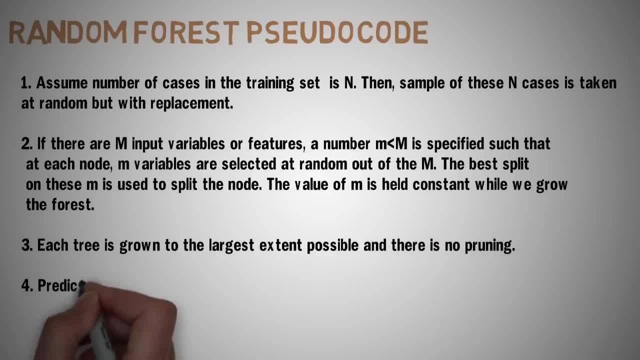 The best split on these M input variables is used to split the node. The value of M is held constant while we grow the forest. Each tree is grown to the largest number. The tree is grown to the largest extent possible and there is no pruning. 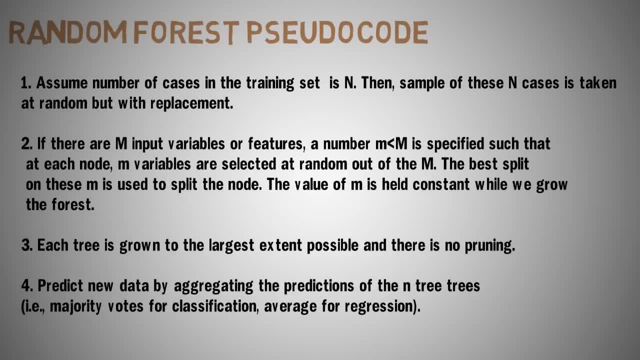 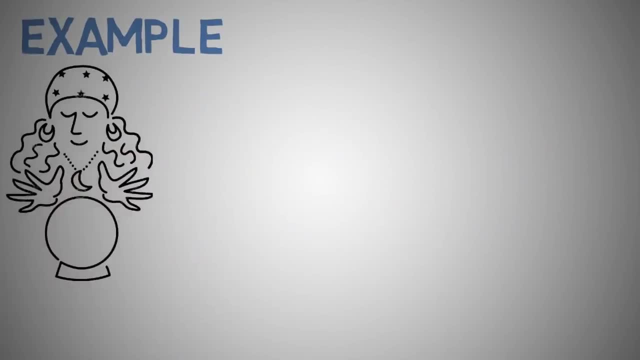 Then we predict the data by aggregating the predictions of the N trees, Which means majority vote for classification and average for regression. So to perform the predictions using the trained random forest algorithm, we need to pass the test features through the rules of each randomly created tree. 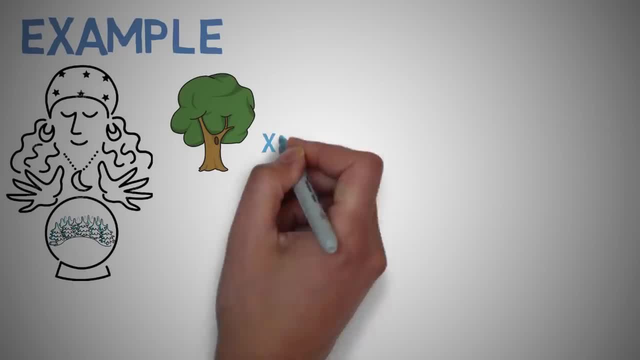 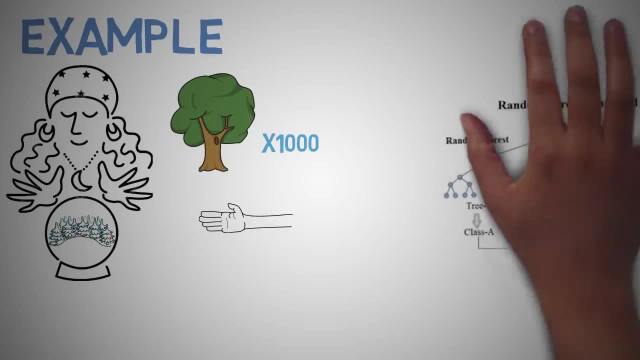 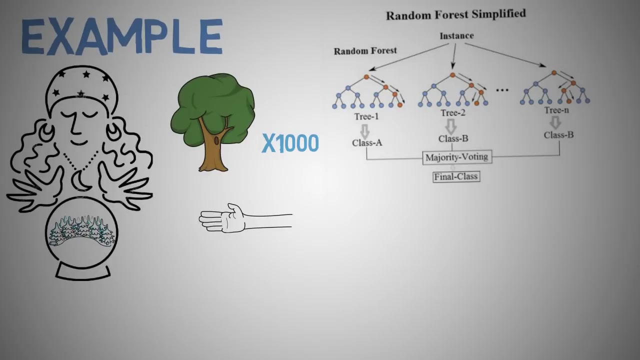 Suppose, let's say, we formed a thousand random decision trees to form the random forest They will be detecting if an image contains a hand. Each random forest will predict a different outcome or class for the same test feature. A small subset of the forest will look at a random set of features, for example a finger. 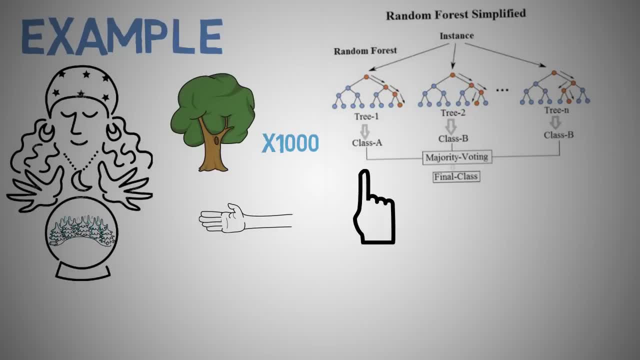 Suppose, 100 random decision trees predict some 3 unique targets such as a finger, thumb or maybe the male. Then the vote of a finger is tallied out of 100 random decisions and likewise for the other two targets. If finger is getting highest votes then the final random forest returns the finger as. 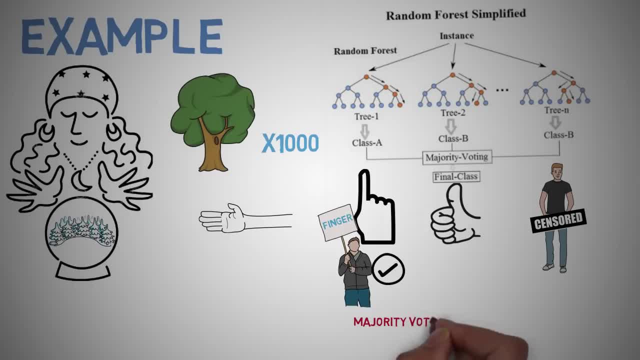 a predicted target. This concept of voting is known as majority voting. just like elections, The same applies to the rest of the fingers of the hand. If the algorithm predicts the rest of the fingers to be fingers, then the high level decision tree can vote that. the image is a hand. 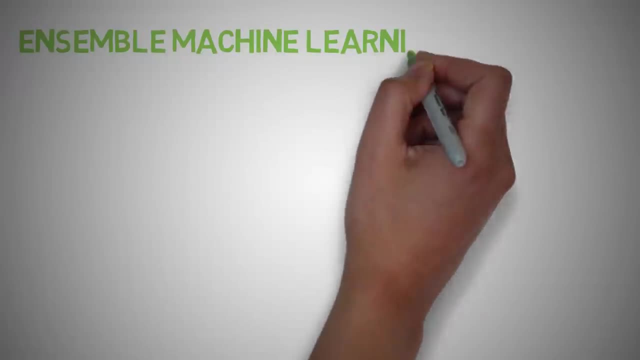 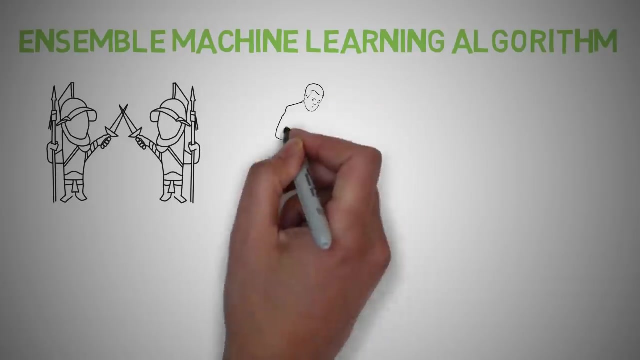 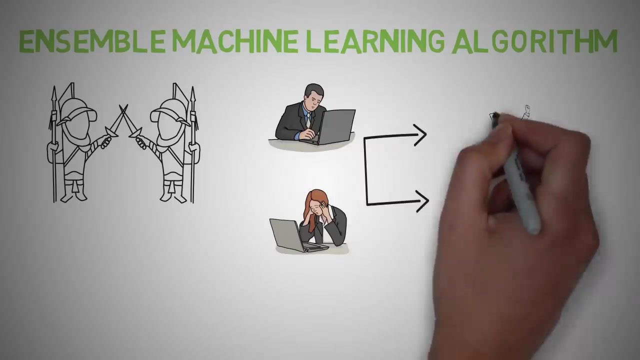 And this is why random forests are known as Ensemble Machine Learning Algorithm. Ensembles are a divide and conquer approach used to improve performance. The main principle behind ensemble methods is that a group of weak learners can come together to form a strong learner. Each classifier is individually a weak learner, while the classifiers taken together are a 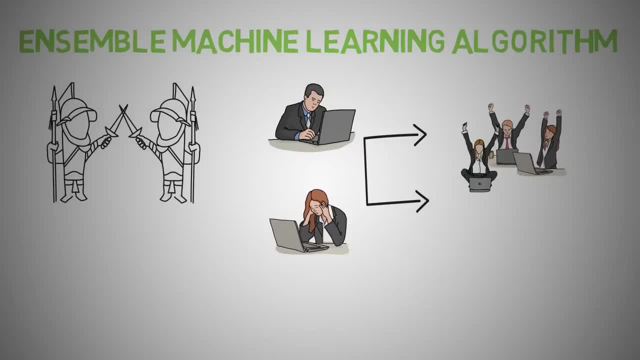 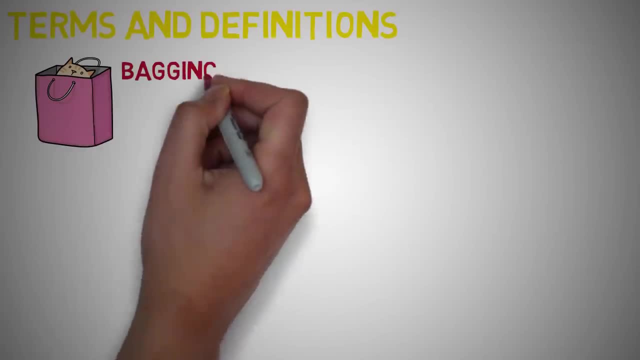 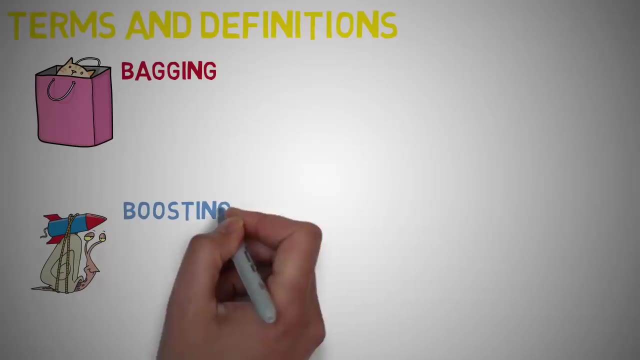 strong learner And thus ensemble methods reduce the variance and improve performance. Before we end the lecture, let's take a look at some terms and definitions that you might come across, such as bagging and boosting. Bootstrap aggregating is also known as bagging, which is a machine learning ensemble meta-algorithm. 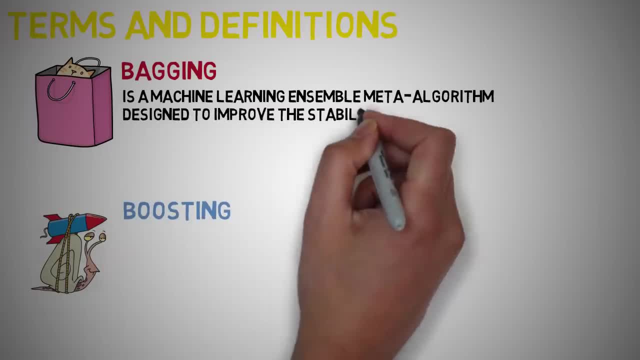 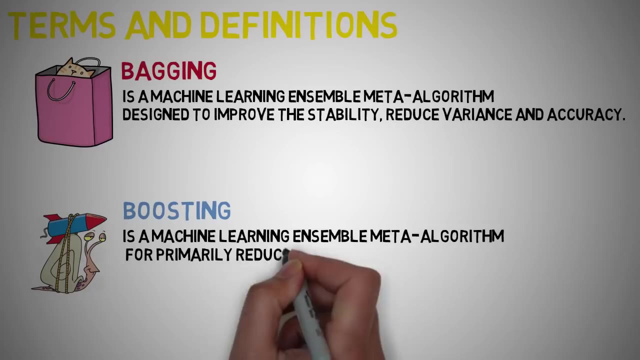 designed to improve the stability and accuracy of the machine learning algorithms used in statistical classification and regression. It also reduces variance and helps to avoid overfitting. Boosting is a machine learning ensemble meta-algorithm for primarily reducing bias and also variance in supervising 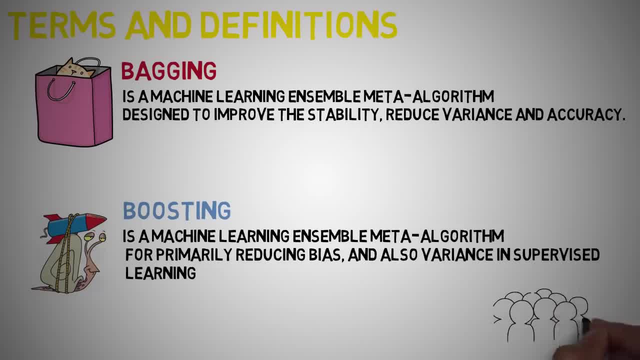 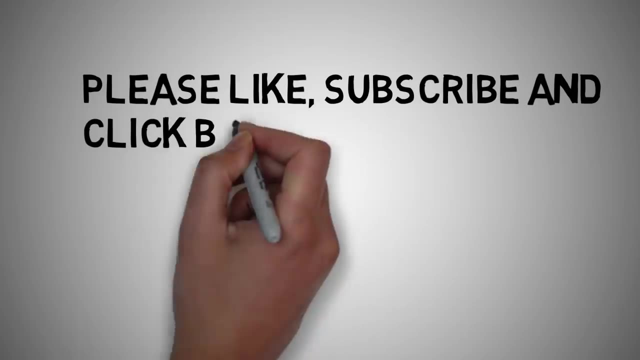 And a family of machine learning algorithms which also convert weak learners into strong ones. Algorithms that achieve hypothesis boosting quickly become simply known as boosting. Okay, so that is it. thank you for watching. please don't forget to like, subscribe and share. Click that bell icon to get notified of more fun and easy machine learning algorithms. 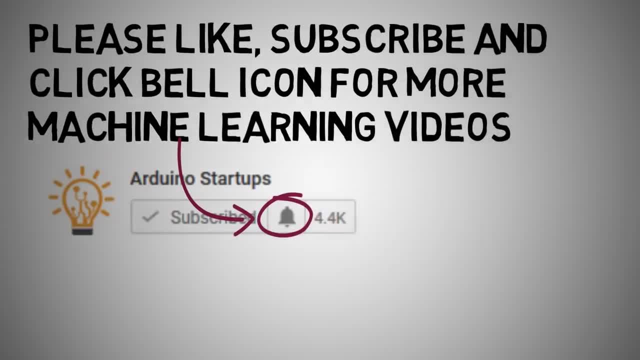 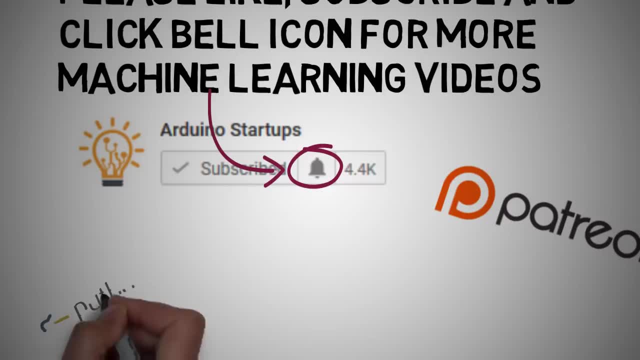 Also, animating these videos takes a lot of time and effort, so please don't forget to support us on Patreon. In the following lecture, we will learn how to implement a simple random forest in python. See you in the next lecture. thank you for watching.